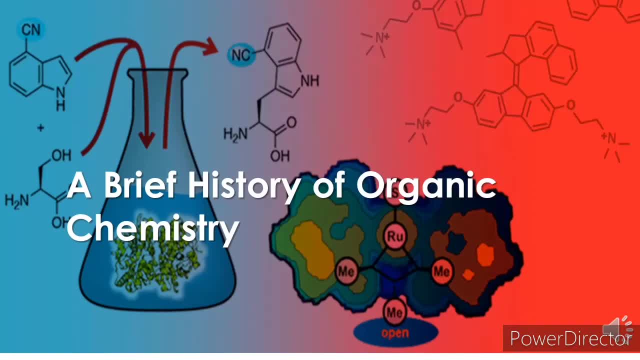 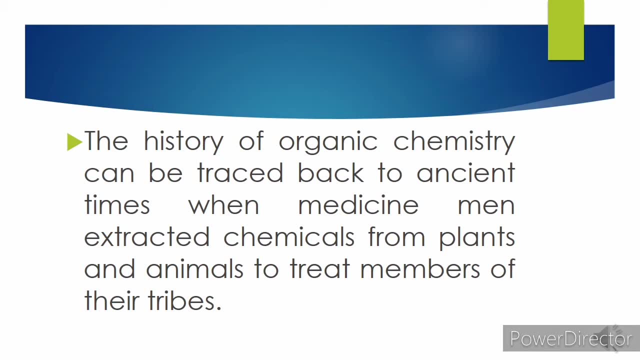 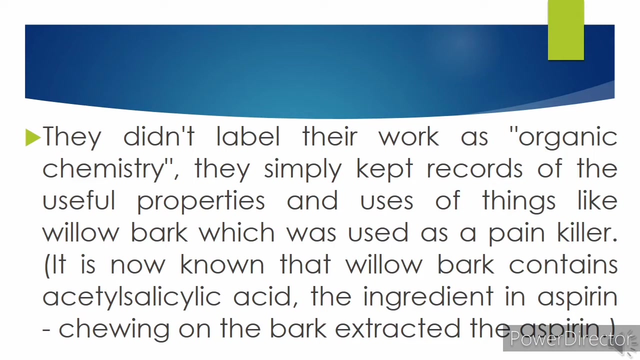 A Brief History of Organic Chemistry. The history of organic chemistry can be traced back to ancient times, when medicine men extracted chemicals from plants and animals to treat members of their tribes. They didn't label their work as organic chemistry, They simply kept records of the useful properties and uses. 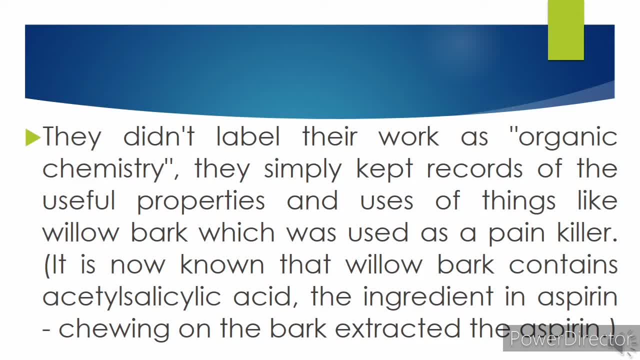 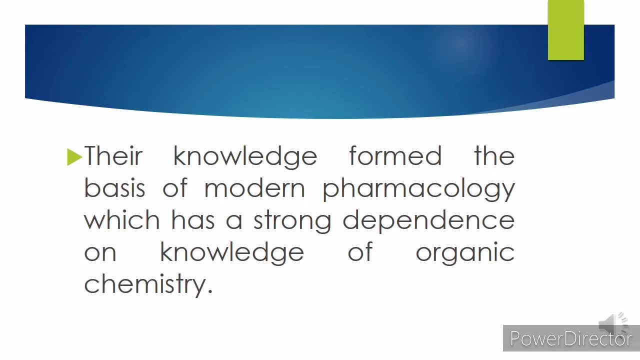 of things like willow bark, which was used as a painkiller. It is now known that willow bark contains acetyl acilic acid, the ingredient in aspirin. Chewing on the bark extracted the aspirin. Their knowledge formed the basis of modern pharmacology, which has a strong dependence. 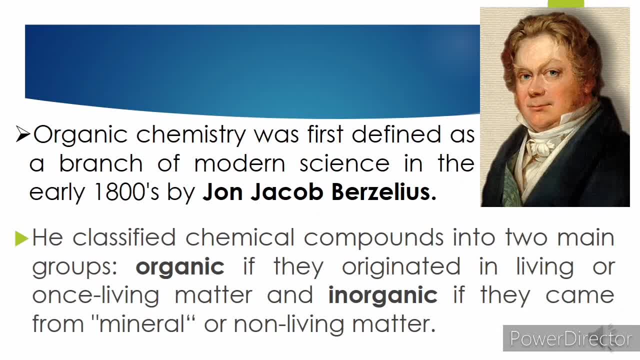 on knowledge of organic chemistry. Organic chemistry was first defined as a branch of modern medicine. All the chemical compounds in the body were made up of organiclichen oins. Although all the chemical compounds in the body were made up of organic root, Although, 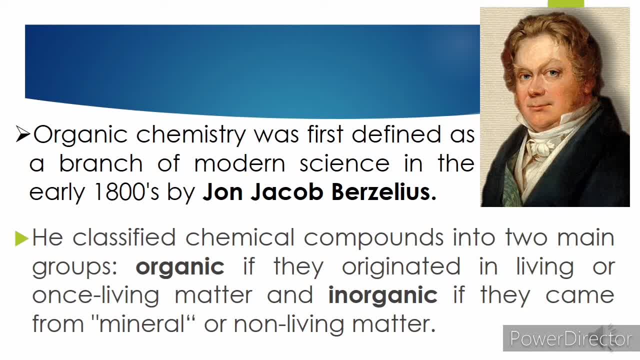 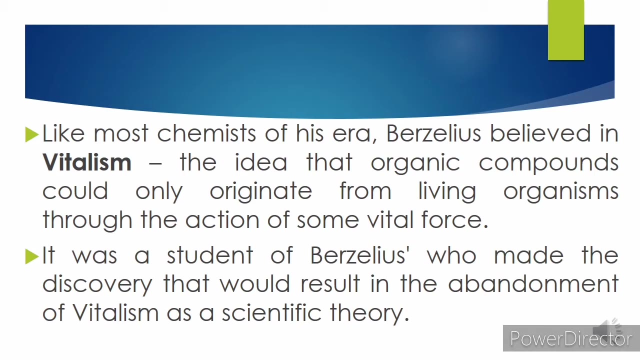 science in the early 1800s by John Jacob Berzelius. He classified chemical compounds into two main groups: organic, if they originated in living or once living matter, and inorganic, if they came from mineral or non-living matter. Like most chemists of his era, Berzelius believed in vitalism, the idea that 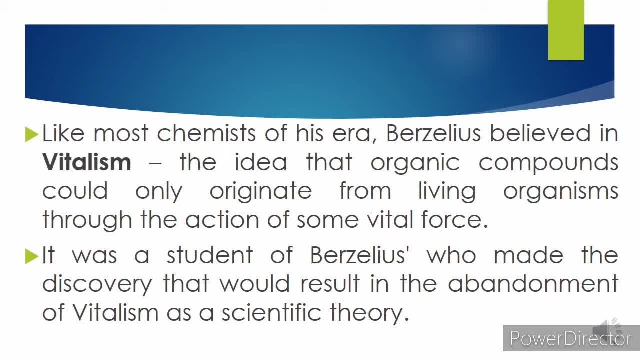 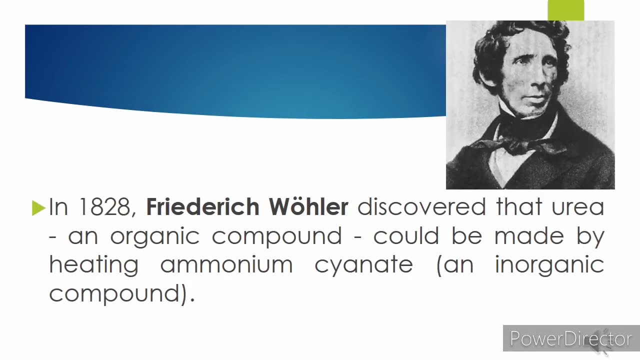 organic compounds could only originate from living organisms through the action of some vital force. It was a student of Berzelius who made the discovery. that would result in the abandonment of vitalism as a scientific theory. In 1828, Friedrich Wöhler discovered that urea, an organic compound, could be made by 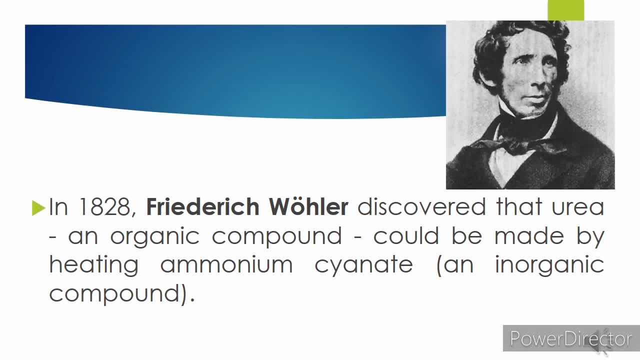 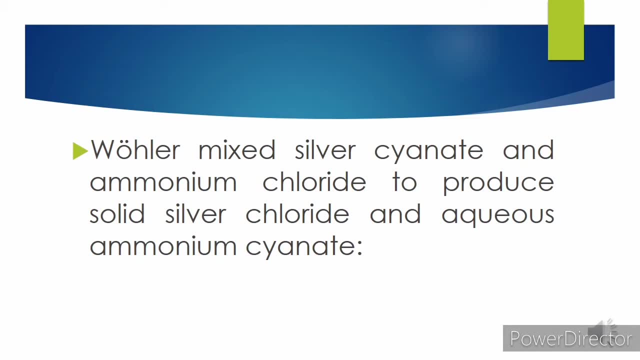 heating ammonium cyanide, an inorganic compound. In 1828, Friedrich Wöhler discovered that urea, an organic compound, could be made by heating ammonium cyanide, an inorganic compound. Wöhler mixed silver, cyanide and ammonium chloride to produce solid silver. 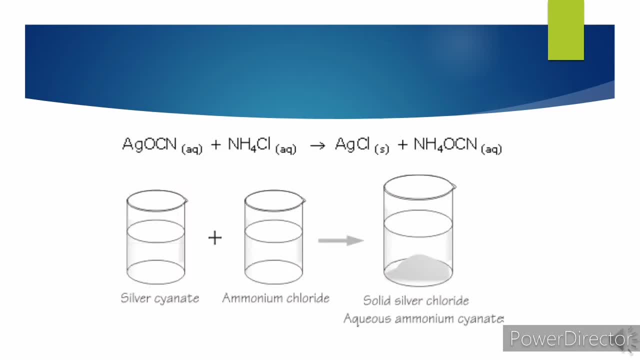 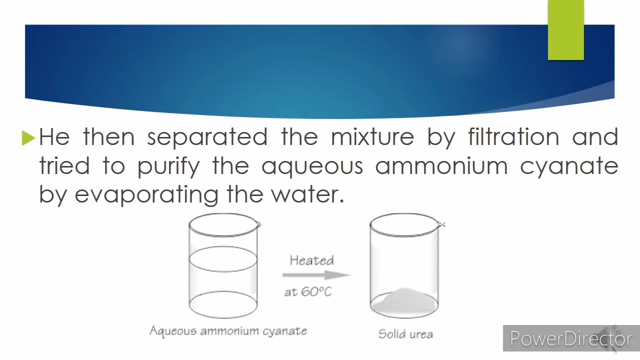 chloride and aqueous ammonium cyanide. This is the chemical reaction of silver cyanide and ammonium chloride that will result to silver chloride and ammonium cyanide. He then separated the mixture by filtration and tried to purify the aqueous ammonium cyanide. 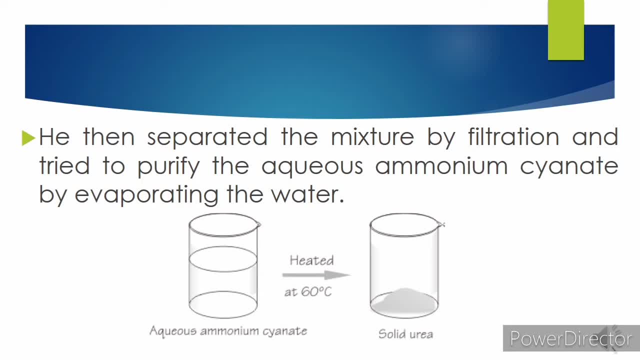 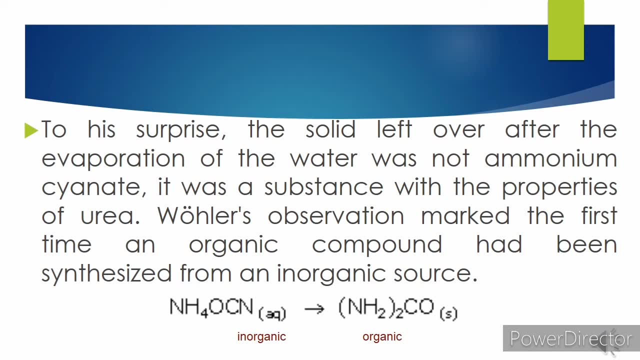 He then separated the mixture by filtration and tried to purify the ammonium cyanide by evaporating the water. To his surprise, the solid left over after the evaporation of the water was not ammonium cyanide. it was a substance with the properties of urea. 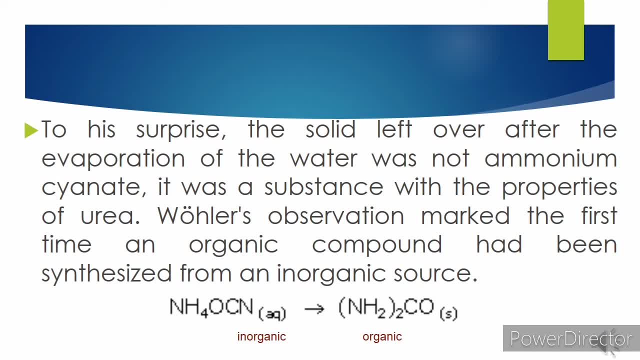 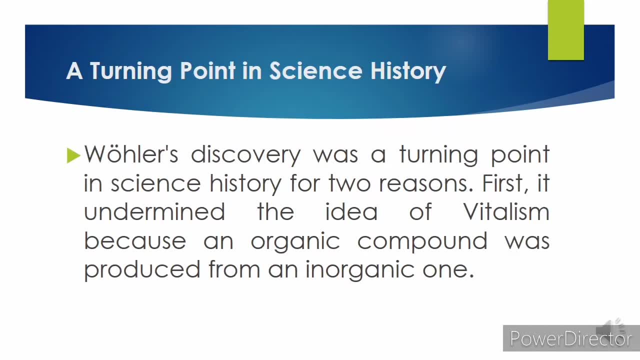 Wöhler's observation marked the first time an organic compound had been synthesized from an inorganic source- A Turning Point in Science History. Wöhler's discovery was a work of past discovery. Wöhler's discovery was a work of past discovery. Wöhler's discovery was a work of past discovery. 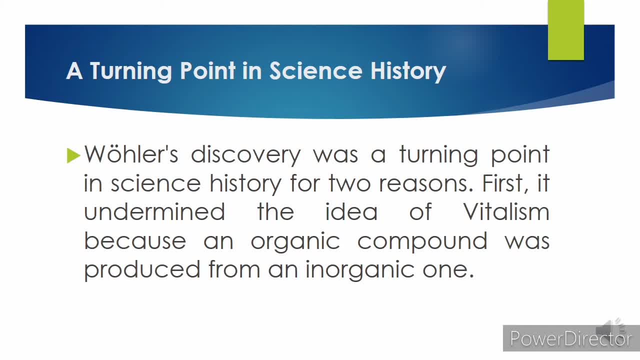 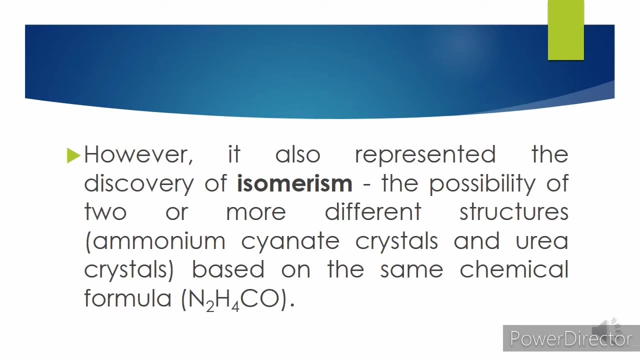 was a turning point in science history for two reasons. First, it undermined the idea of vitalism, because an organic compound was produced from an inorganic one. However, it also represented the discovery of isomerism, the possibility of two or more different structures. 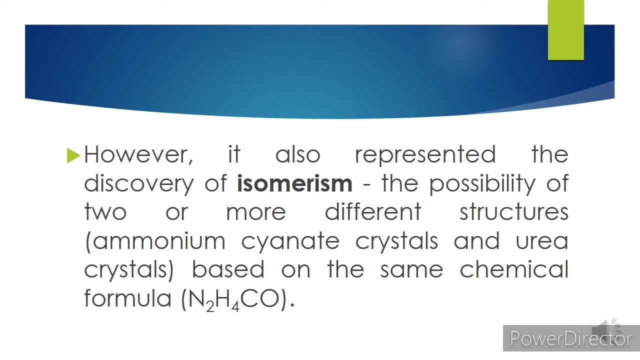 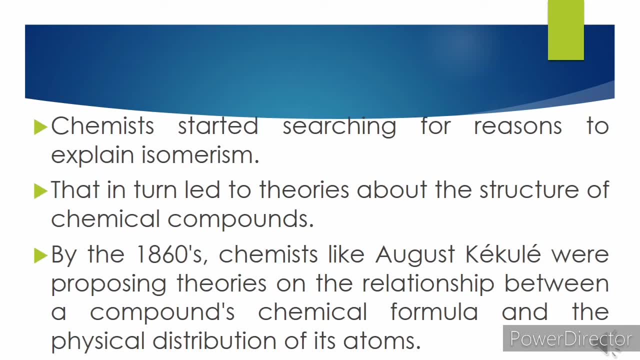 based on the same chemical formula, Chemists started searching for reasons to explain isomerism. that in turn led to theories about the structure of chemical compounds. By the 1860s, chemists like August Kekulé were proposing theories on the relationship between a compound's chemical formula and 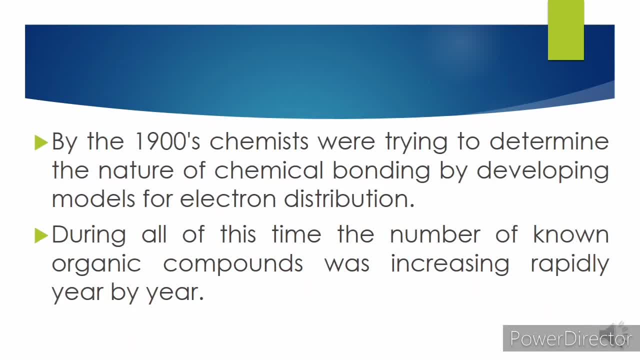 the physical distribution of its atoms. By the 1900s, chemists were trying to determine the nature of chemical bonding by developing models for electron distribution. During all of this time, the number of known organic compounds was increasing rapidly year by year. During the 20th century, organic chemistry 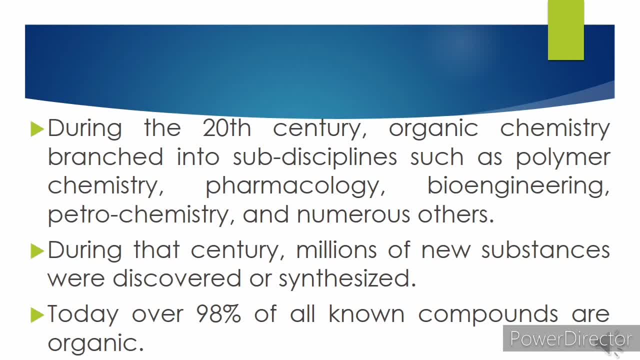 branched into sub-disciplines such as polymer chemistry, pharmacology, bioengineering, petrochemical engineering and chemical engineering. During that century, millions of new substances were discovered or synthesized. Today, over 98% of all known compounds are organic.